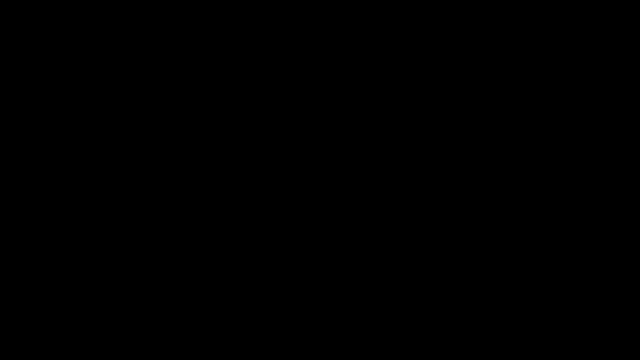 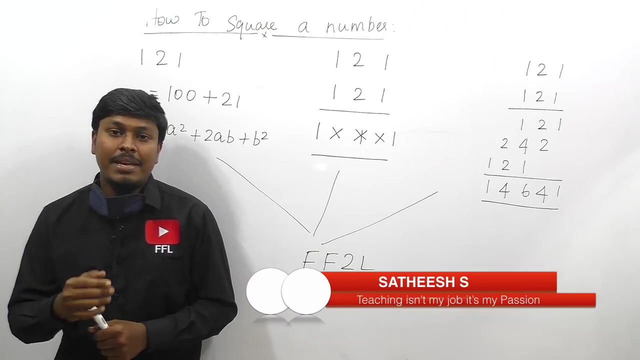 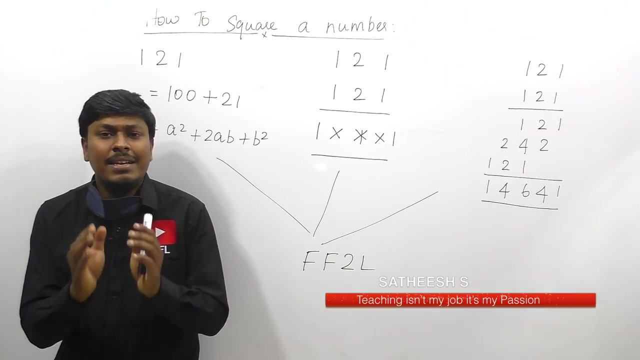 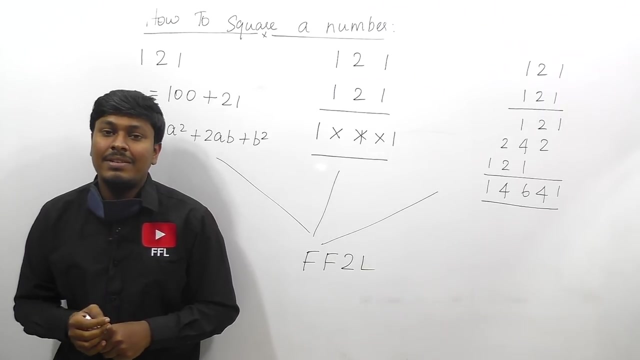 Hello, friends, first of all, thanks for being here in my YouTube channel, and today we are going to see how to square a number faster. So, friends, everybody, intention is to square a number faster, right that too? in a competitive exam, we need to square a number within five seconds. So, friends, 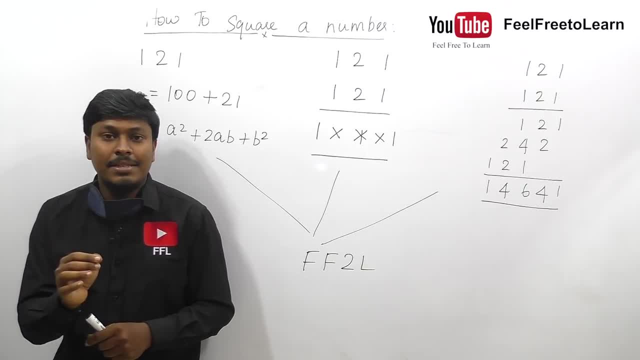 I am just going to teach you a right method and a faster method and a smarter method to square a number. So, friends, if you are preparing for a competitive exam, if you are not going to any institution, then you will surely know this first method right, which we learned from the 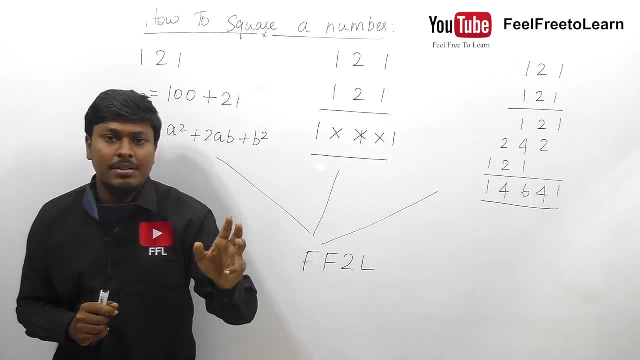 schoolings right. Second method: if you go for any institution, then they will teach one cross, a three cross, that is, cross one, in order to solve the squaring a number faster. If you search many YouTube videos, then you can surely say that this method is nowadays most of the student is applying. 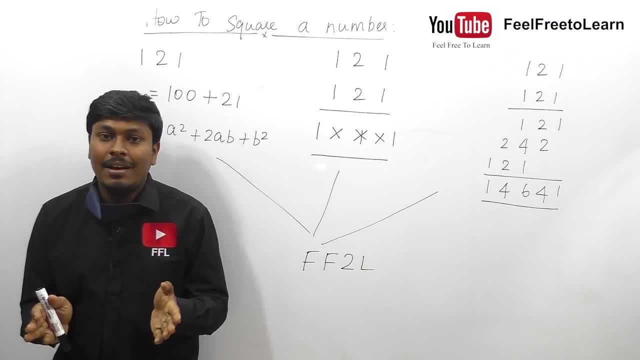 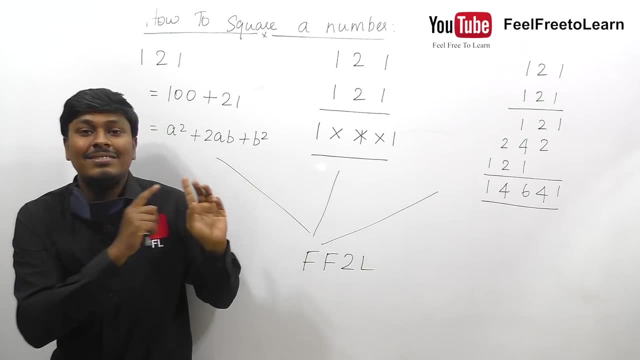 that is a square plus two, a b plus b square. So, friends, I am not at all going to teach you a magic, right, I am just going to teach you a best method by using all these three method friends. Why? because in the first method I have just found what is the drawback when we use this method in 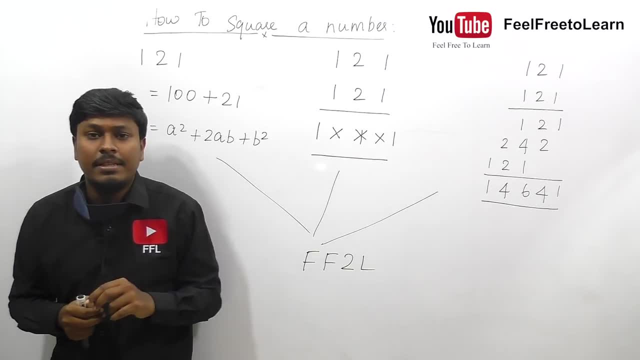 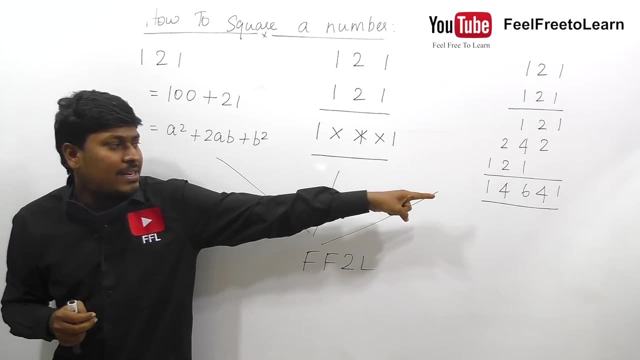 the competitive exam. I just found out what are the drawbacks of this three method. First method: the main drawback is it takes me, takes just more than one minute. right, if it is a 992 square, definitely it will take more than one minute. And this method, where I think it is a universal 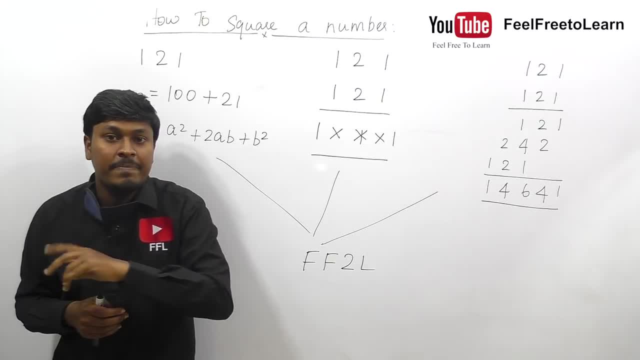 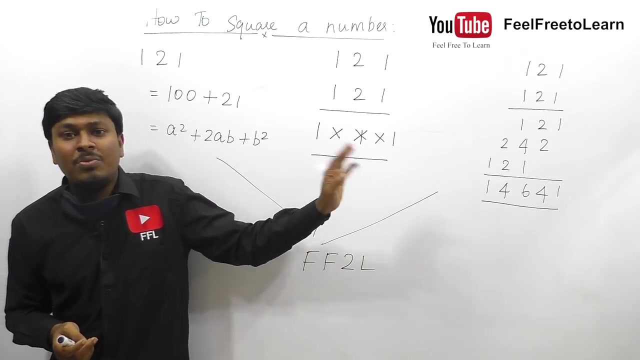 method. So I can say that this method is applied for a smaller number, right? so 121,, 131,, 108, we can use this number. If it is a huge number, like 777, 773, then surely this method takes you more than. 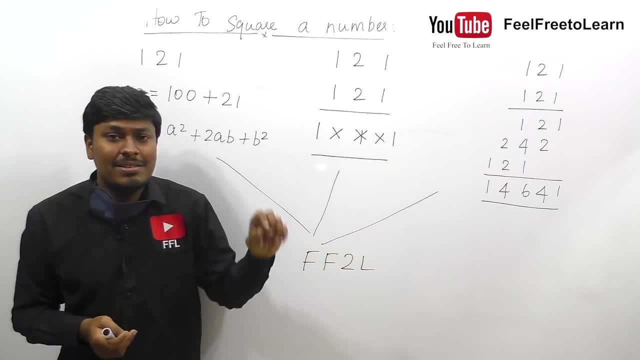 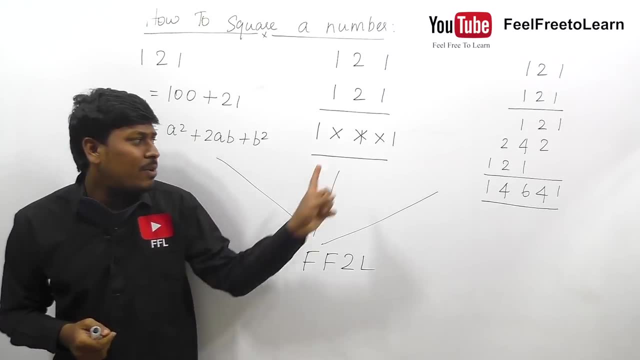 one minute when compared to that method, friends. Why? because we need a huge addition. we need to add 42,, 33,, 43, something like that. we should properly add all the values. So I can surely say that I won't suggest this method to any of my students. So I am not going to suggest this method. 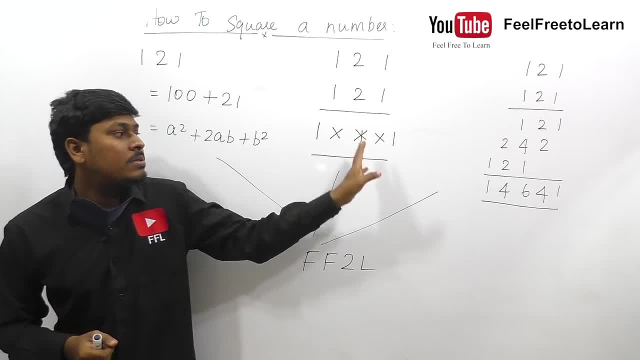 to any of my students. So I am not going to suggest this method to any of my students. So I am not my friends. I only think is that don't follow this method. better follow this method, or better follow this method. don't follow this method why? because it requires. 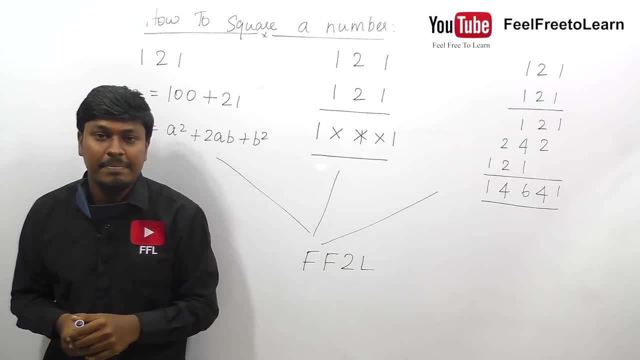 a huge addition, friends. definitely we will make a mistake in the exam. And the third method which is recently followed by many students, that is a formula a-square plus b-square plus to AP. this method is applied for a easy number if it is in the range of 200-300, but if it is in the range of 400. 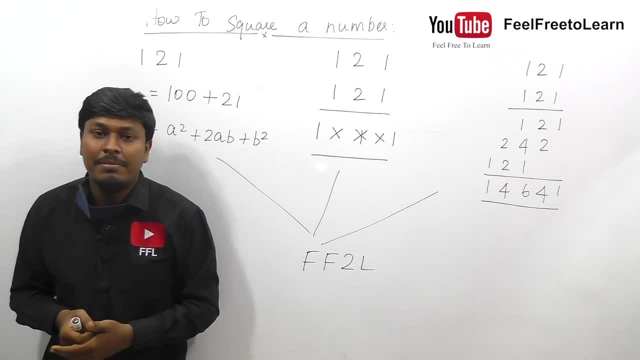 or 500, we can't able to use this method. definitely, this also takes you one minute. So, friends, I have just found out what are all the drawbacks- drawbacks of this three method. and finally, I have found my method in my YouTube channel. surely you will love it, surely you will enjoy it. no doubt about it. but my only advice: practice more than 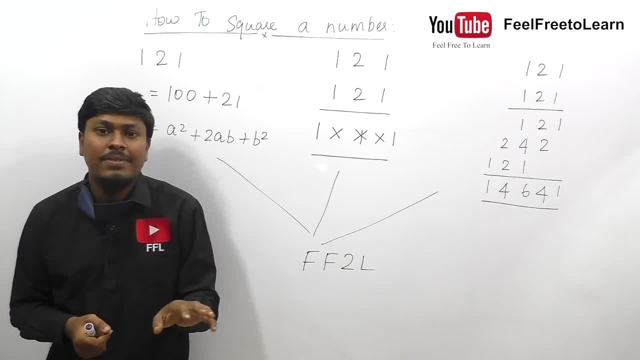 one month. just by seeing this video you can't able to square a number faster. practice a lot and lot. at least 50 to 100 number, friends, so that you can surely crack equation in an exam. you are just going to learn a new method. just download this video, share this video to all your friends, so 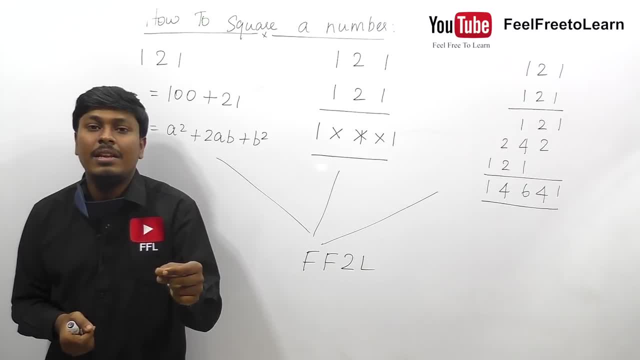 that your friends can also learn. download this, keep it safe on your laptop or a mobile phone, practice daily a minimum of two or three numbers. I will surely say that you will be so brilliant than me. so, friends, let me move on to the excellent method now. so, friends, before applying the technique, 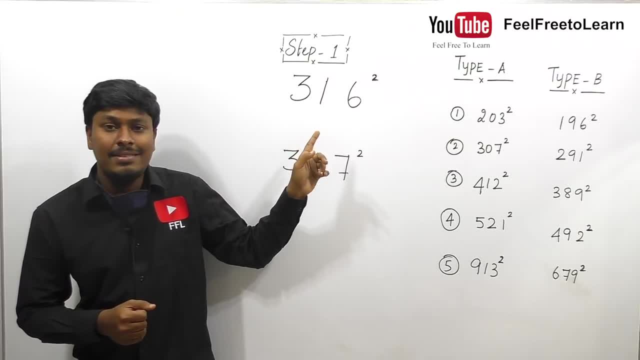 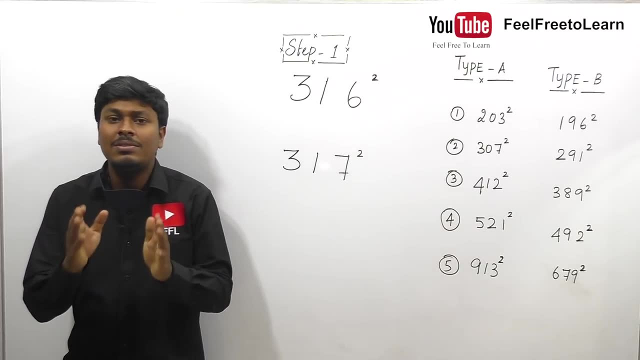 you should note two important thing: what is the difference between 3- 16 square and 3: 17 square, and why this number is called as type A and why those number is called as type B? you should know this. two important concept, friends. first of all, we see what is the difference between. 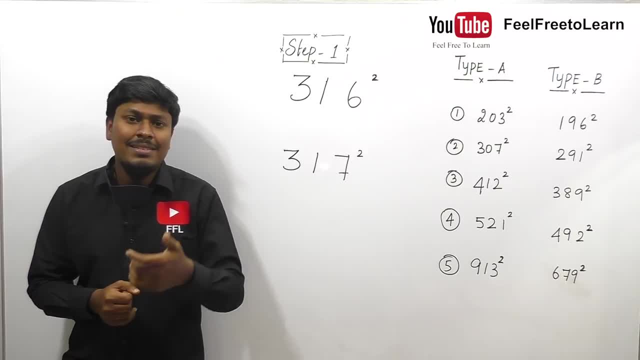 3- 16 square and 3- 17 square. so, friends, just kindly take your calc and see what is 3- 16 square. if you square this 3- 16, the answer will be 9, 9, 8, 5, 6. if you square 3- 17, then the answer will be 1 0- 0 then. 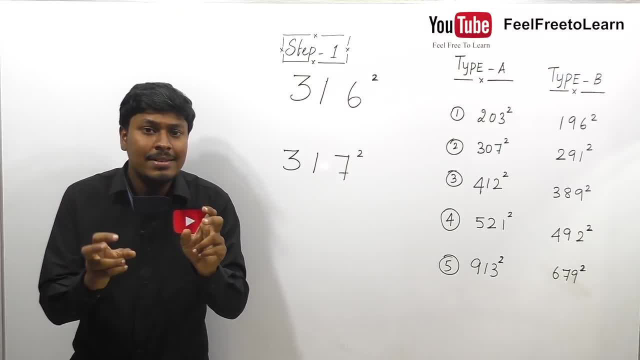 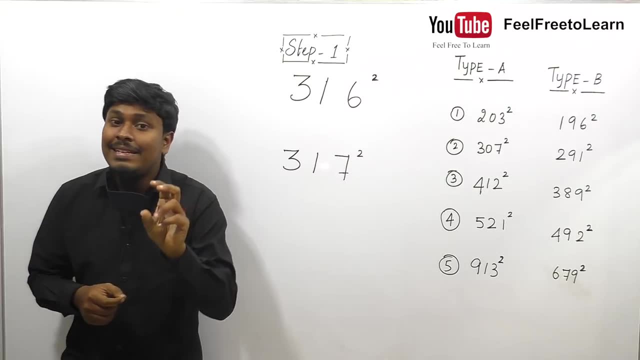 4- 8, 9. so, friends, when you keenly watch the answer, what is the difference between 3- 16 and 3- 17? so, friends, the 3- 16 square answer is 5 digit, 3- 17 square and 3- 17 square. so, friends, when you keenly watch the answer. what is the difference between 3- 16 square and 3- 17 square? the answer is 6 digit. so from this we can clearly say that from 100 till 3- 16, when you square any number, the answer should be 5 digit. from 3- 17 till 9- 9- 9, if you square any number, the answer should be 6 digit. friends got. 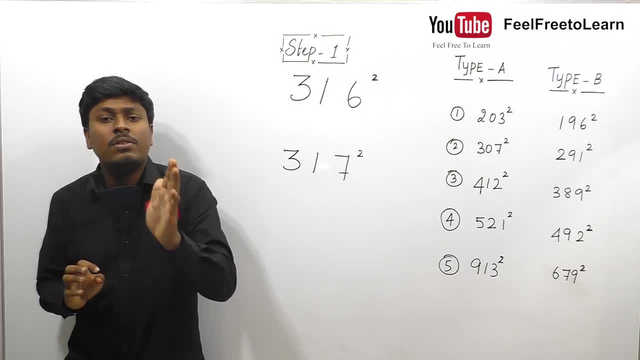 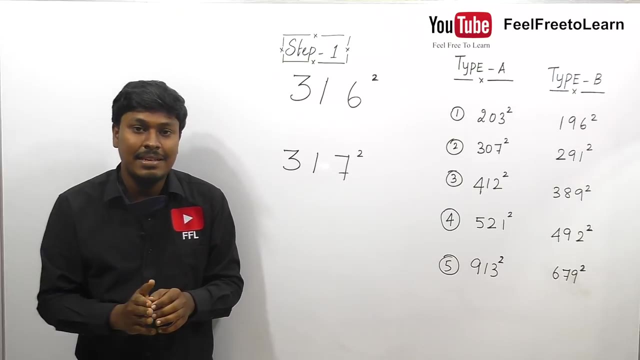 the logic friends, if I am saying, when you what is the answer for 291 square, 291 square, step number 1, you should say whether the answer is 5 digit or 6 digit. I can surely say that the answer should be 5 digit. why? because 291 square is less than 3: 16. if a number is less than 3- 16, then definitely. 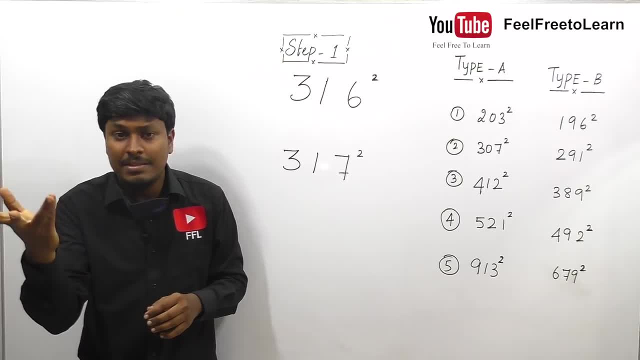 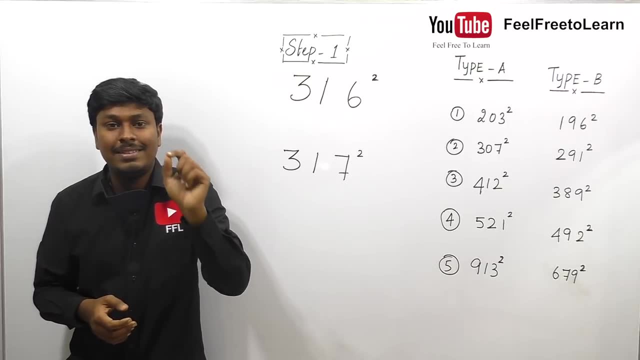 the answer should be 5 digit. if I am saying what is 5 12 square, the number is more than 3- 17, then definitely you should say that the answer should be 6 digit. so this is the difference between 3- 16 and 3- 17. if they are giving any numbers, step number 1, always see whether it is below 3, 16 or. 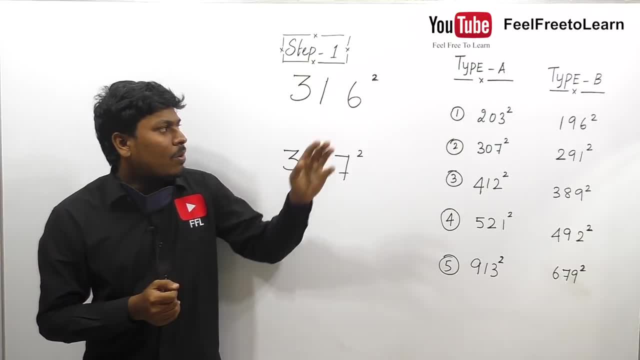 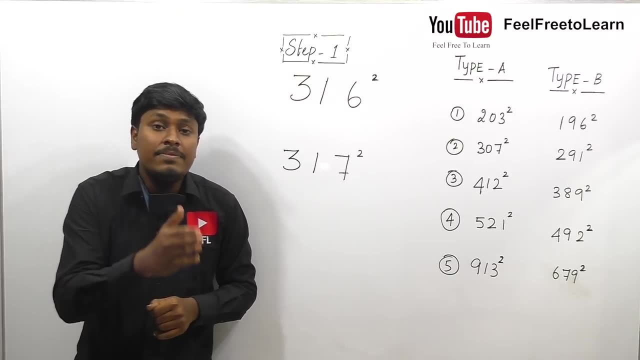 whether it is about 3, 17, right? ok, friends, what is called as type B and type B? friends, listen carefully- between 1 to 50 is called as type A. if a number is from 51 to 100, then it is called as type B. this 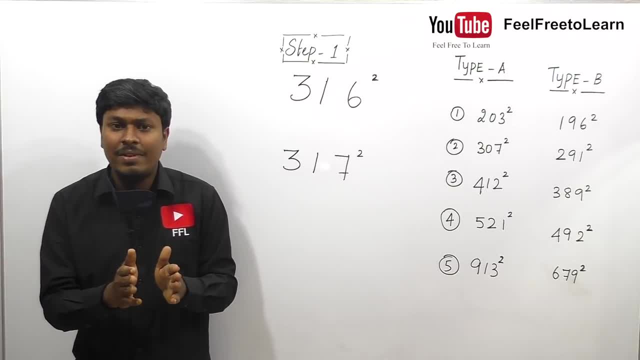 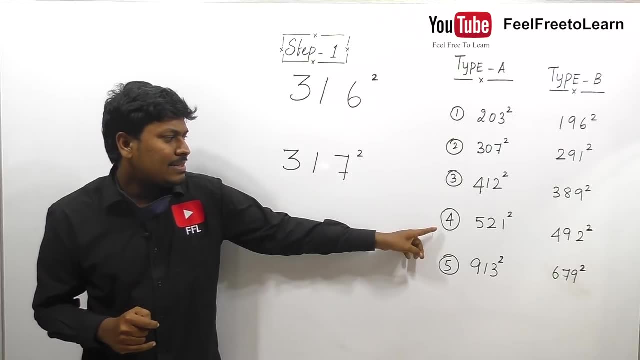 is called as type A and type B, right, there is not a huge difference in solving, but you should remember that why this number is called as type A and why this number is called as type B. for an example, just see 521 square 521 is in the range of 500 to 550, right, when you see, when you any other number, 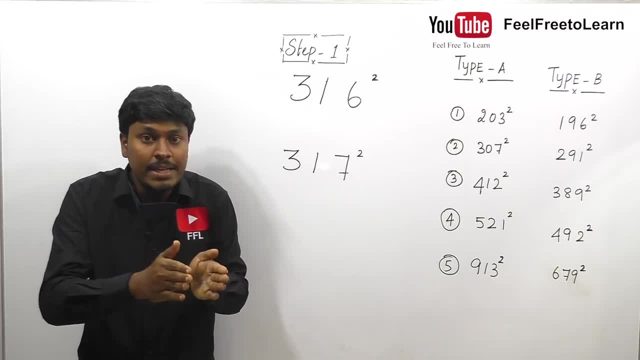 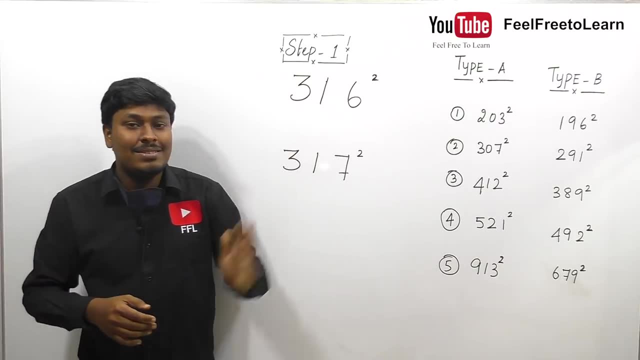 friends, let me see 291. 291 is in the range of 250 to 300. friends got the logic: 1 to 50 is called as type A. if it crosses 51 to 100, then it is called as type B. so, friends, by seeing the, 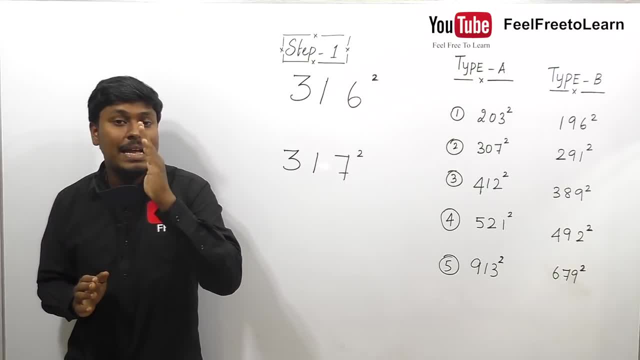 question, step number 1: you should say whether it is 5 digit, whether the answer is 5 digit or whether the answer is 6 digit. step number 2: whether the question whether the number that we are going to square is type number A or type number B. if you know this- two things- you can close. 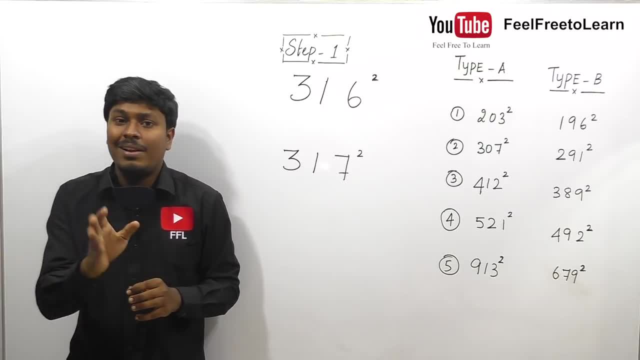 your eyes and say any square right, any square friends. but only thing: by looking at this video, you can't able to say: right, you should practice a lot. minimum of one month, you should practice. so, friends. I took more than three months to practice this, from 100 till 999 square. I took. 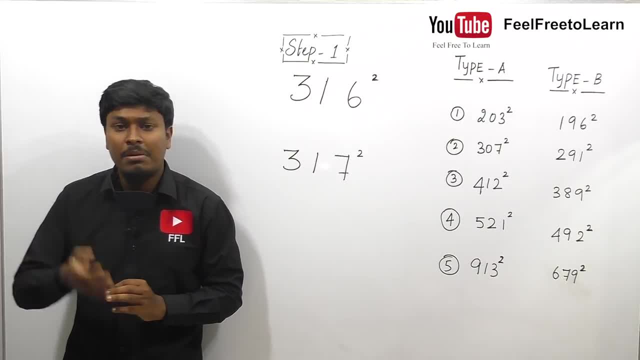 three months, more than three months. I took to square a number by closing my eyes. so, friends, I think you are more brilliant than me. kindly practice more than one month. just concentrate on the smaller numbers, then go for the huge numbers, right? so, friends, let me move on to the 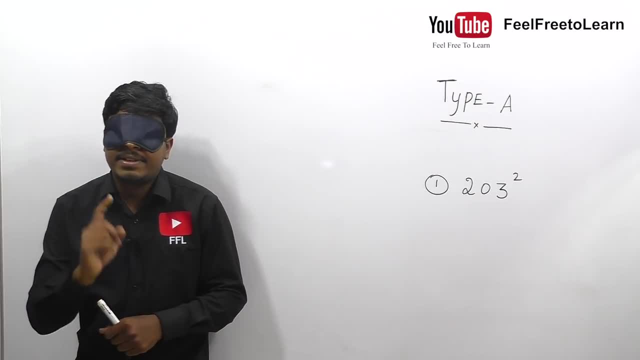 best technique never seen. now let me move on to type number A. the first question, that is, 203 square, is the number that is between 1 to 50, right? so 203, 205, 230, wherever the number that is 1 to 50. that 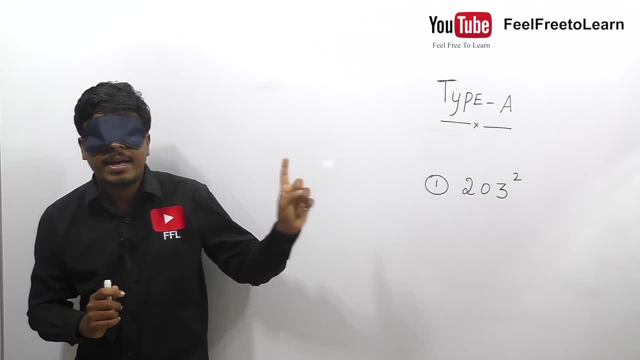 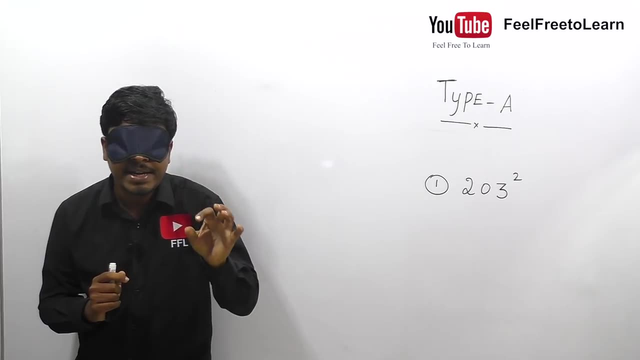 is called as type number A. so, friends, now our target: to square a number, that is 203, step number 1. always remember that by seeing a number itself, you should say whether the answer is 5 digit or whether the answer is 6 digit. by seeing a number, I can surely say that the answer is 5 digit you. 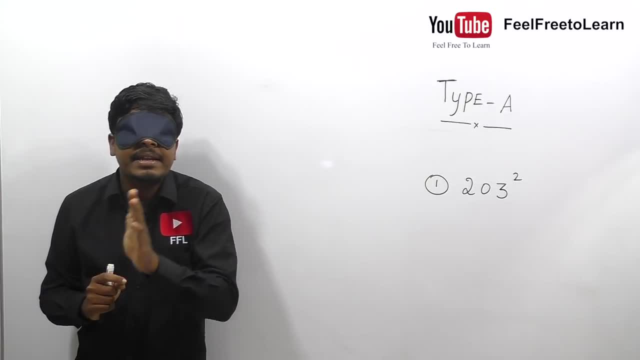 know that in the basic itself I have told you, if a number that is between 100 to 316, then definitely the answer must be 5 digit. here the number is 203. it is definitely below 316, so I can surely say that the answer must be definitely a 5 digit. so, friends, if I, if someone is asking what is 203, 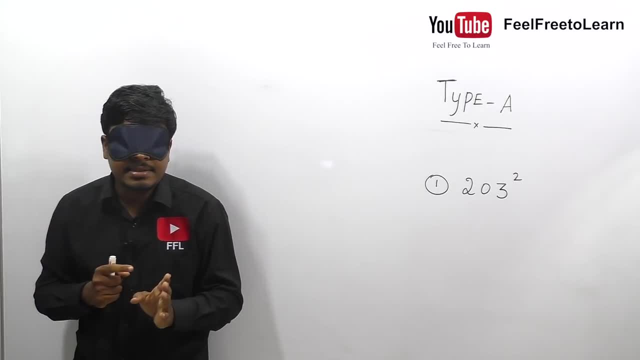 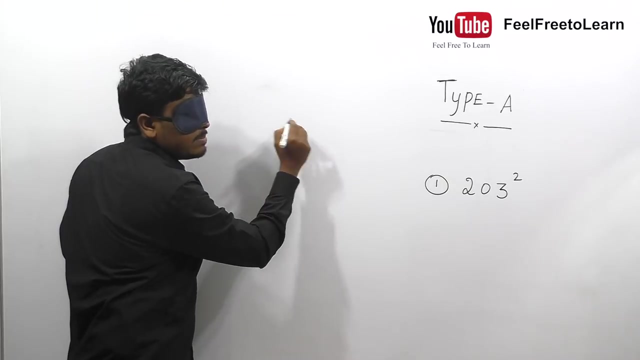 square. I just think for a second and I can say the answer is 4, 1, 2, 0, 9. so this is the answer for 203 square. so, friends, how my mind works. if someone tells any number how my mind works, listen here, friends. 203 square. just listen, listen carefully, friends, I am just going to teach you slowly. 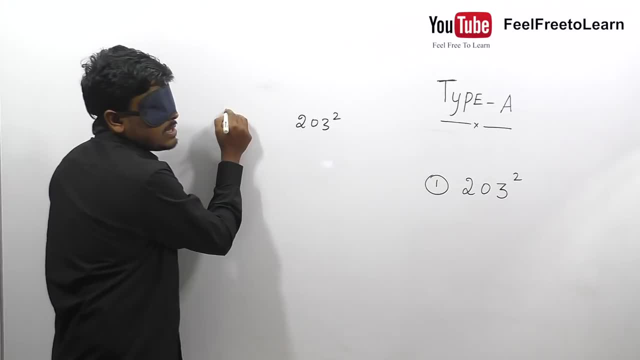 203 square. just listen, listen carefully, friends. I am just going to teach you slowly the first number: 203 square. so, friends, from 200, this happens. i am just taking 200 as a base number from 200. we need to find what is 203 square from 200. it is not. three more friends got the point. 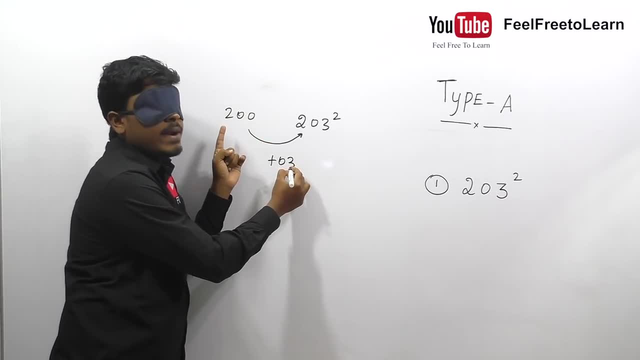 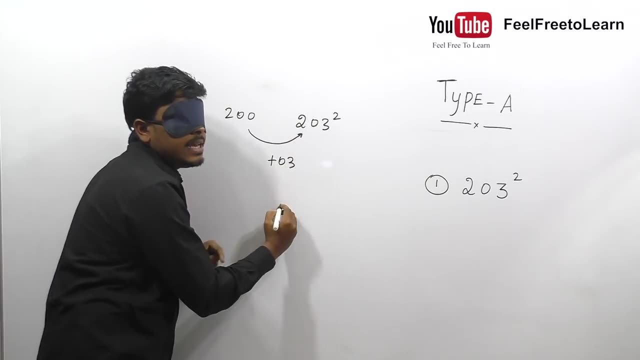 our target to square a number 203. i am just taking 200 as a base number from 200. it is not three more, right? i am just going to add not three again to the same number. that is, 206, friends. got the point, friends, right? i am just going to add not three again to the same number. now we got 206. we took. 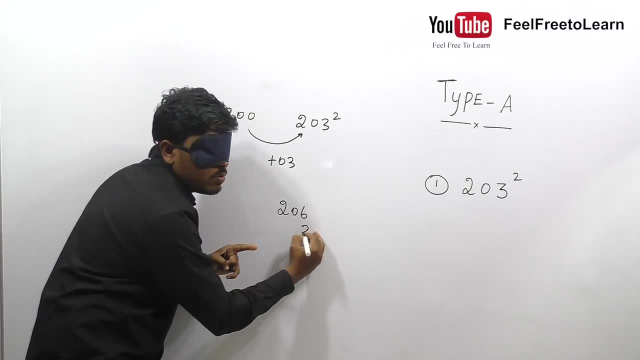 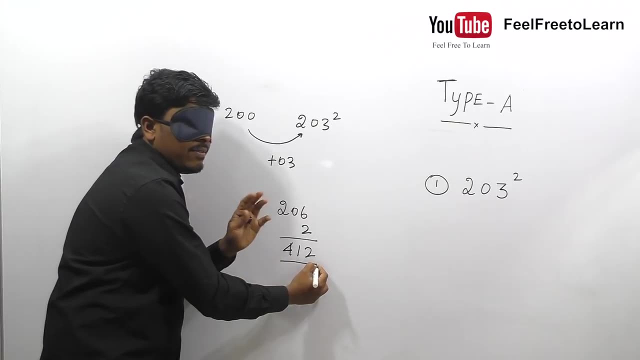 200 as a base number. so multiply this 206 by 2, so finally we got 412. since, listen carefully- finally we got 412, which is three digit. so, friends, we already know that if we square 203, definitely the answer must be five digit. now we got 412, three digit. remaining only two digit from 200. 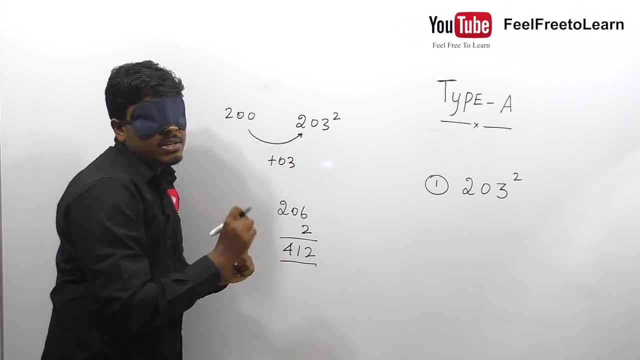 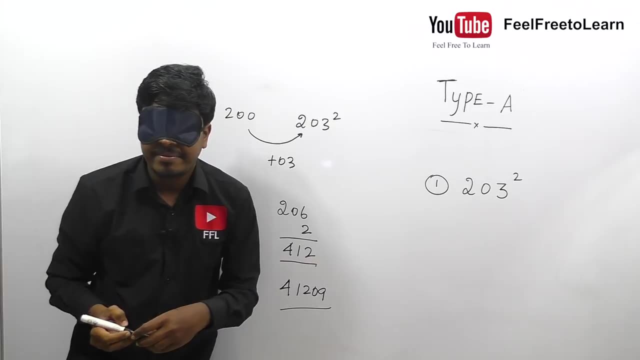 it is three more, so three square will be nine. i can surely say that the answer must be four one, two zero nine. so this is the answer for 203 square. so, friends, this is the way my mind works. if someone tells the number, let's got the point, friends, first. 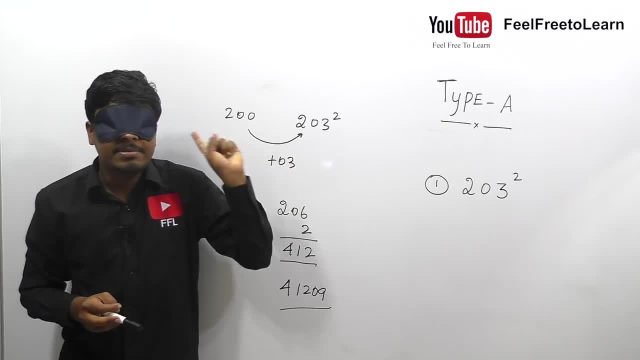 of all our target to square a number that is 203. i am just taking 200 as a base number. from 200 it is three more. so i am just adding, not three again to the same number, that is 206. we took 200 as a. 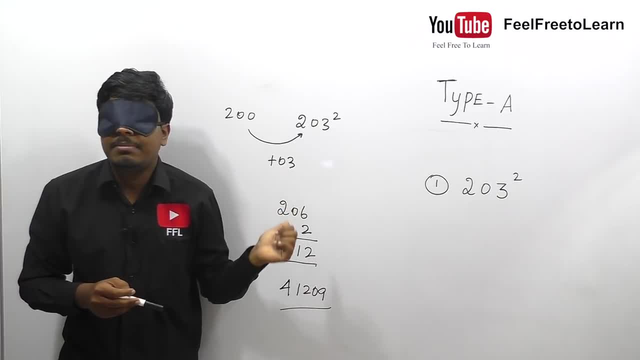 base number. so i am multiplying by two, two or six into two, the remaining will be four, twelve. so, friends, now we got four, one, two. friends- listen carefully- we got three digit. we know that the answer must be definitely five digit. from 200, it is three more, so three square will be nine. so 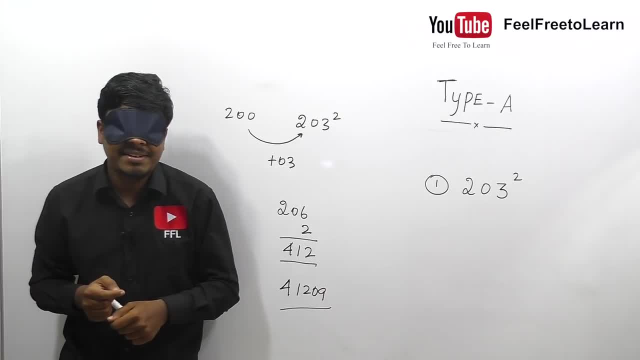 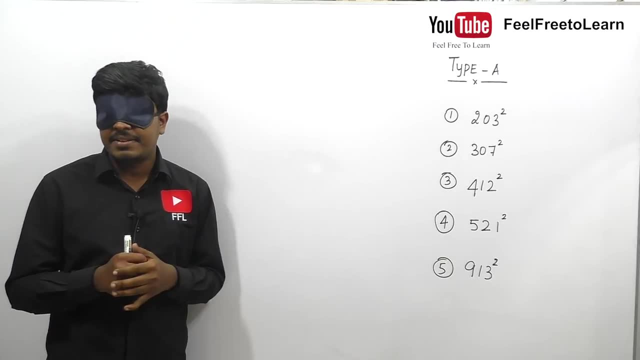 finally, i can say the answer is four, one, two, zero, nine. we square the second number, the second number that is three, not seven, square. so, friends, our target, to square a number that is three, not seven. so step number one, always by seeing a number itself, you should say whether the answer is five. 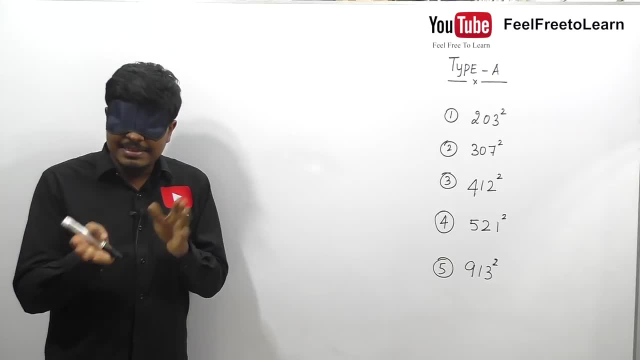 digit, or the answer is six digit. this three, not seven, is less than three sixteen. so i can show you clearly. say that the answer must be definitely five digit number, right? so, friends, in the previous case we can surely say that the answer is in the range of 200, right? the first question is 203 square. 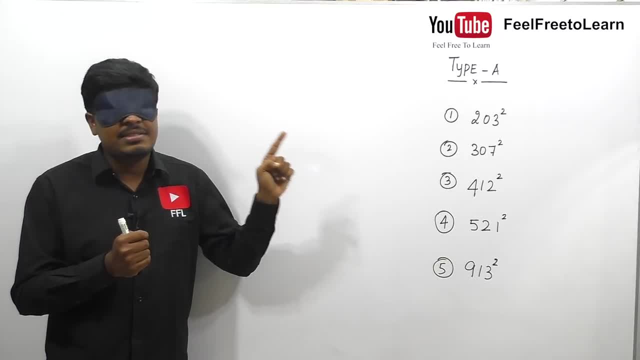 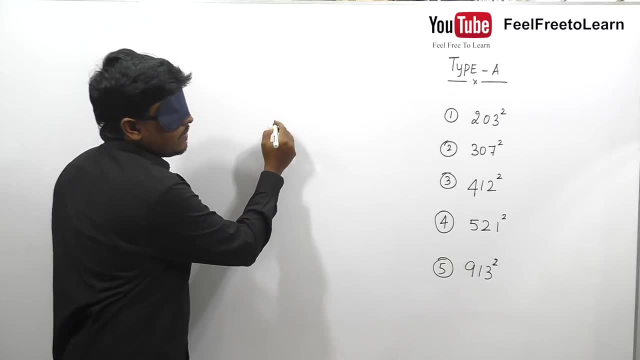 we can say that the number is in the range of 200. but the second question is 307. friends, listen here. the second question is 307, so we can say that the number is in the range of 300. right? so, friends, our target to square a number that is 307 square. i can say that this 307 square, isn't that this? 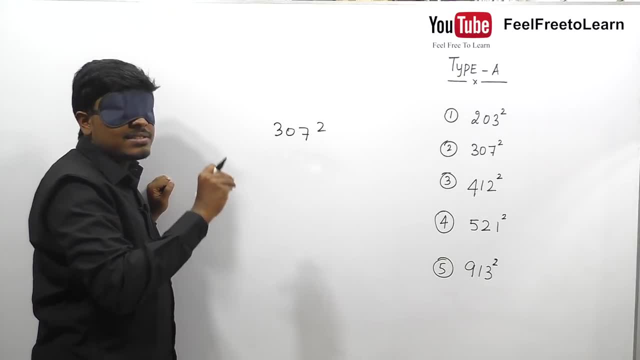 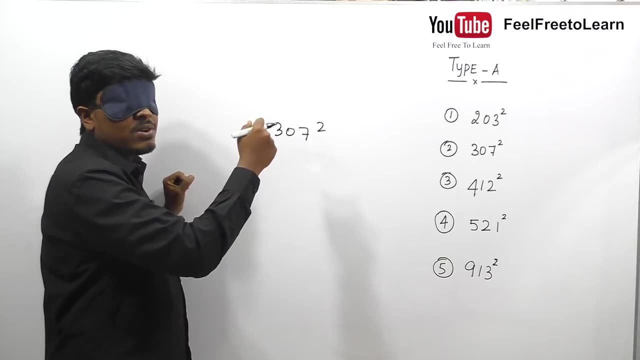 is approximately in the range of 300, from 300. it is 07 more. so i am just going to add 07, that is 07, again to the same number. when we add this 07 again to this 307, then we can got this as 314. so friends, got the logic, what i have. 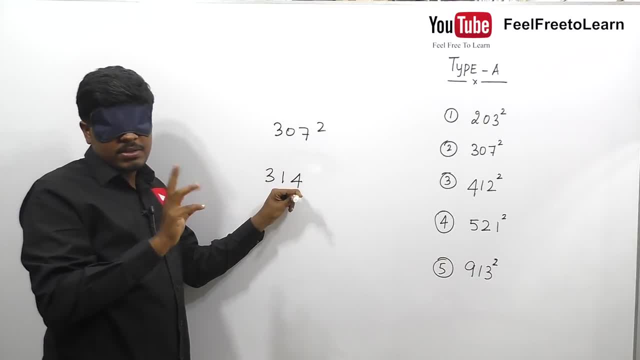 did is just listen, listen carefully, friends. in the previous case it is 2, 1, 2, 0, 3 from 200. it is 3 more right? so i am just adding 03 again to the same number. so that is 206. so here the number is. 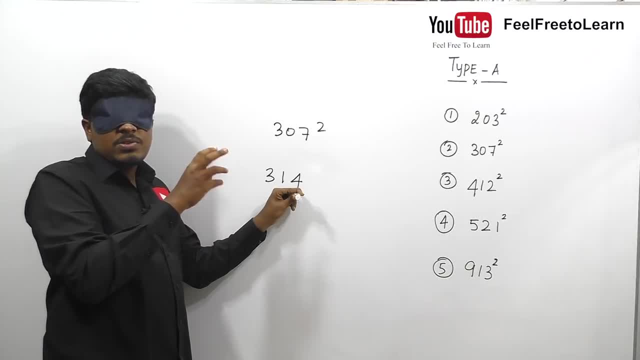 307, right? so it is nearer to 300. so from 300 it is 07 more. so i am just adding 07 again to the same number. so when we add 07 again to the same number, that is 314. so, friends from the previous, 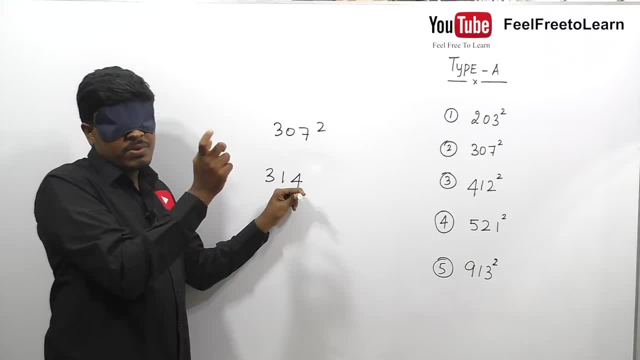 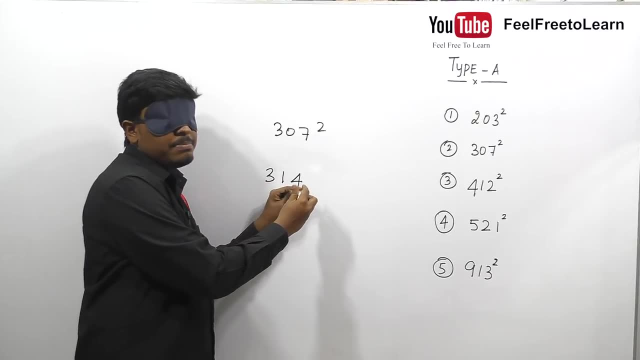 case we have multiplied by 2. why? because it is in the range of 200. but in this case it we need to multiply this number by 3. why? because it is in the range of 300. so when we multiply this, 314 into 3- so friends, listen here- 4 into 3 will be 12. 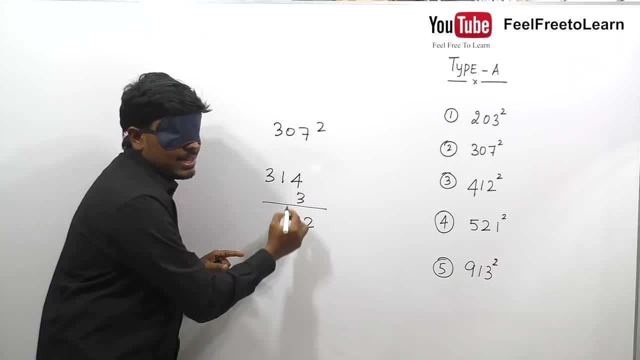 you right. so reminder will be 1. 3 into 1 will be 3, 3 plus 1 will be 4, right? so 3 into 3 will be 9. so, friends, finally, we got 942. so friends, listen here. now we got the answer, that is 3 digit you. 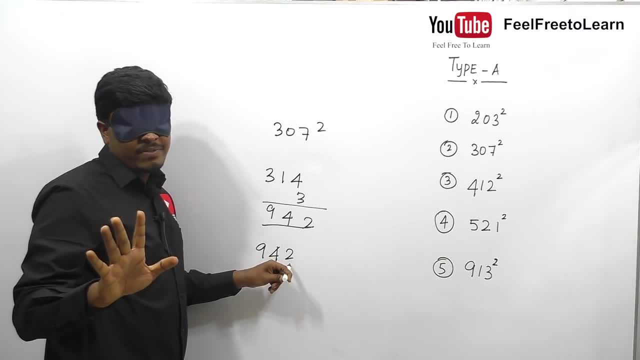 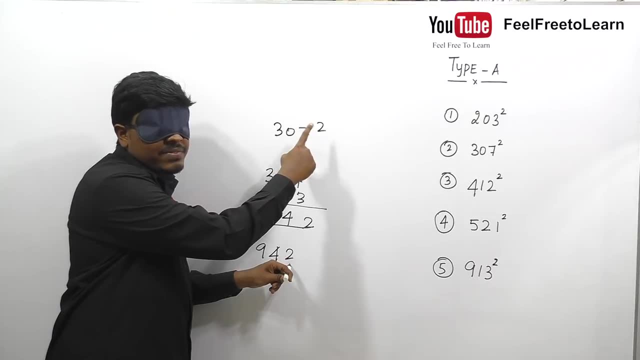 know that when we square 307, definitely the answer should be 5 digit. so only 2 digits are remaining. friends, listen carefully. the given question is 307 square 07. when we square this 07, that is 49, so we can surely say that here it is 942.. 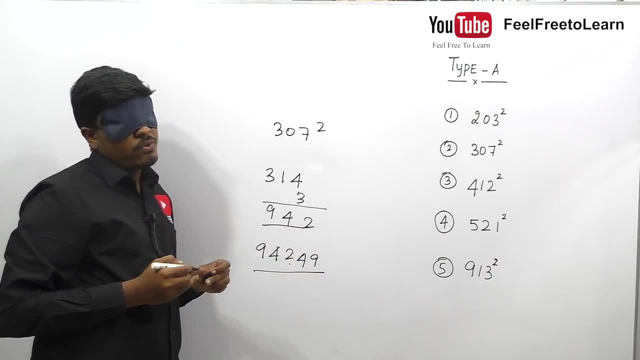 so finally, the answer is 94 to 49. so friends got the logic. what are all the things i have done? step number 1: by seeing a number, whether answer is 5 digit or 6 digit. this is step number 1. this is in the range of 300. so, friends from 300, it is 07 more adding 07 again to the same number. 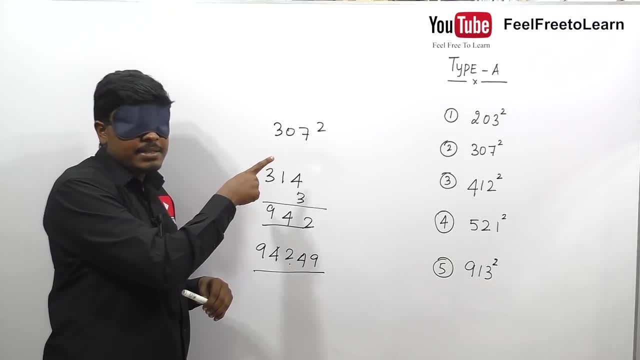 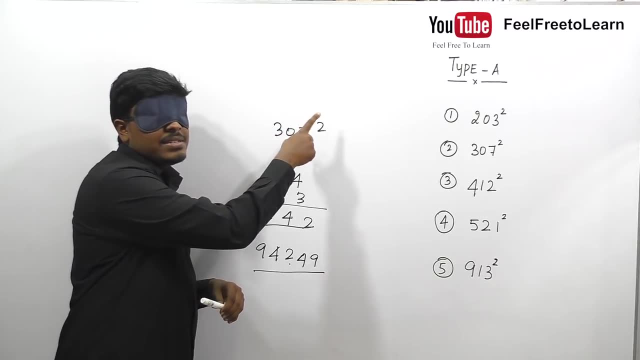 so that is 314, because from 300 we need to multiply this by 3. when we 314 is multiplied by 3, 942, so still we need 2 digit. so the given question is 307 square. when we square this 3, 14. 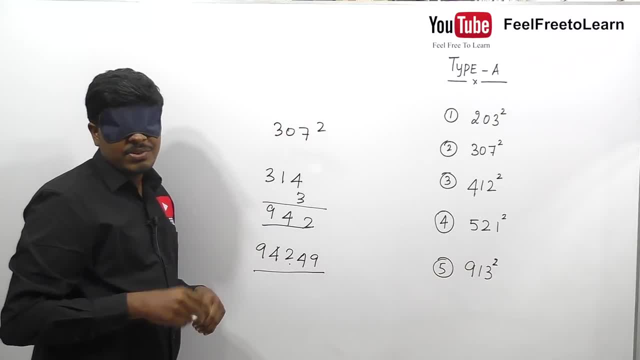 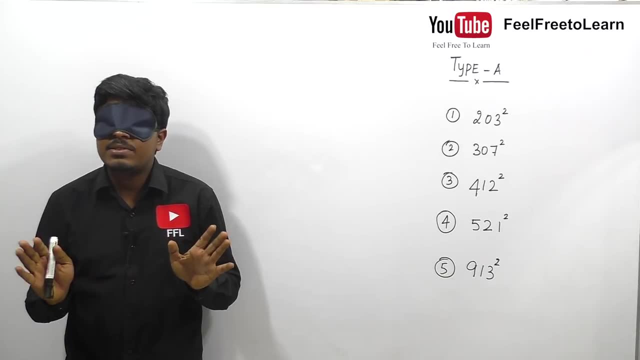 square 07, then 49, so finally we got the 5 digit. so final answer will be 94 to 49. let we move on to the third number, that is 412 square. so, friends, we are just going to square a number that is 412. by seeing a number itself, you should say whether the answer is 5 digit or whether the 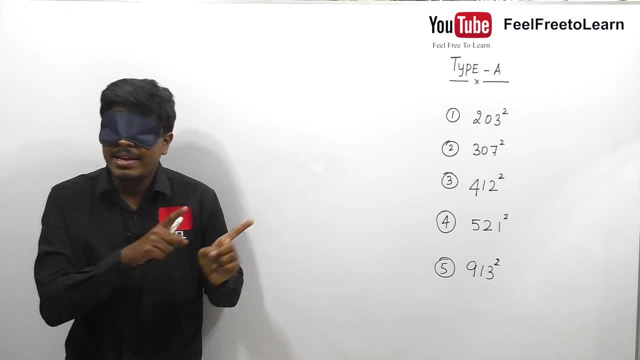 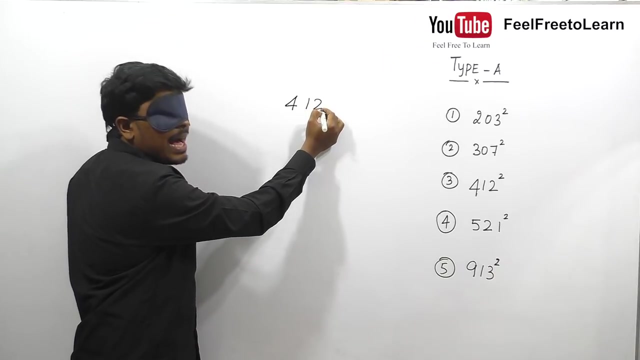 answer is 6 digit. definitely i can say that this number, 412, is greater than 316. if a number is greater than 316, then definitely the answer should be 6 digit. step number 1: so, friends, now our target is 412, right? so friends from 400, it is 12 more. add 12 again to the same number, that is 424. 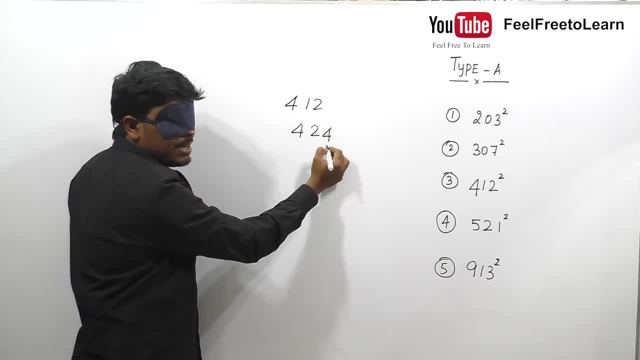 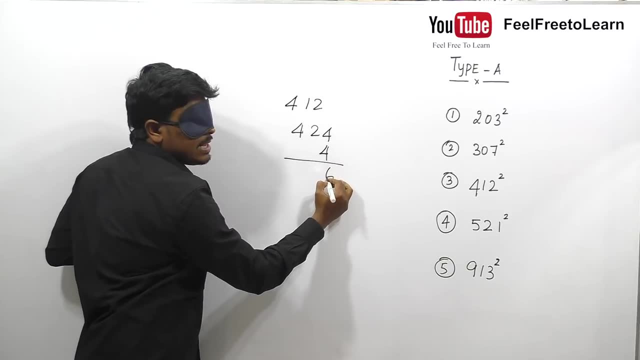 so, friends, in the previous case we have multiplied by 3. in the first case we have multiplied by 2. here it is in the range of 400. so we need to multiply this by 4. so 4- 4s are 16. remainder will be 1. 4- 2s are 8, 8 plus remainder will be 1, that is 9. so 4- 4s are 16. so, friends, finally, we 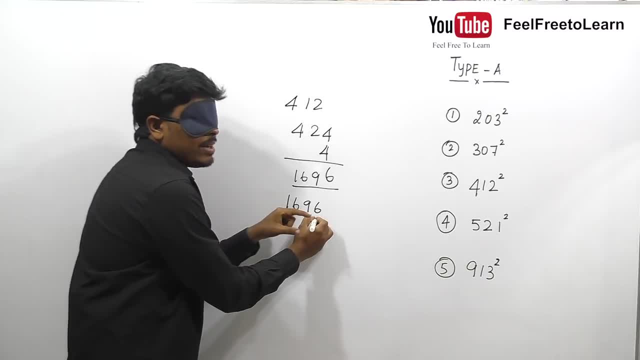 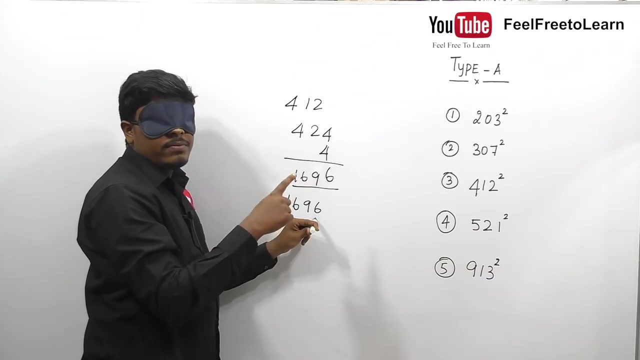 got 1696. listen here, friends, the important step here, right? so finally we got 1696. so, friends, the last two number, or 12. when we square this 12 then 144. if i write 144 here, then the answer will be 1, 6, 9, 6, then 1, 4, 4, but our only target, the answer should be 6 digit. 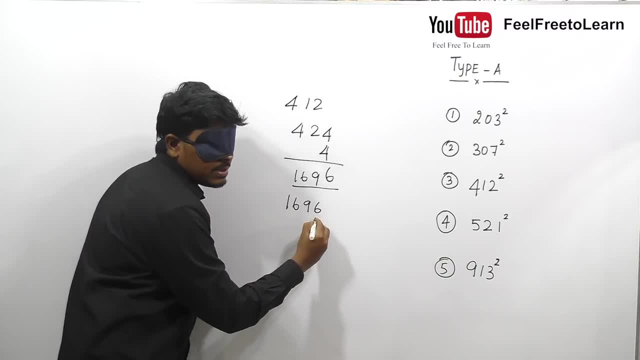 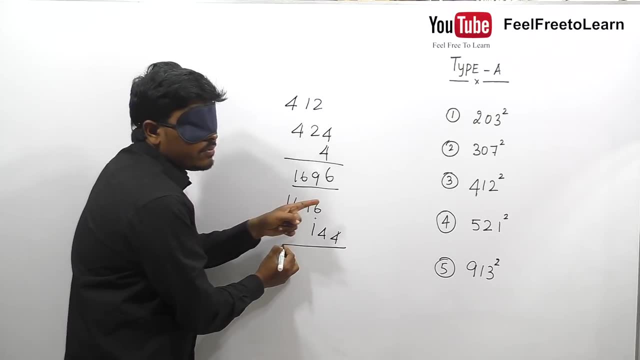 so listen here below 6, friends, listen here below 6. i am just going to write 144, so, friends, got the logic right. so, friends, 12 square will be 144. if i write 144 at the last, then the answer will be 7 digit. but our target, we know the. 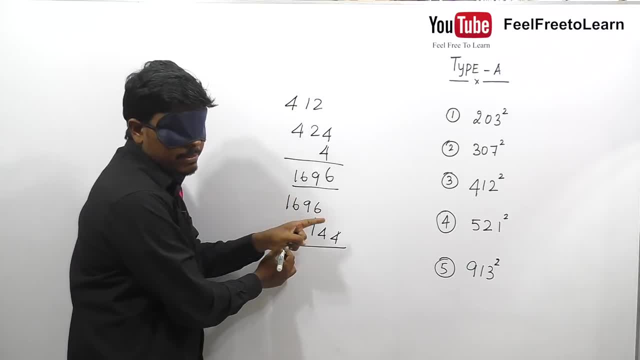 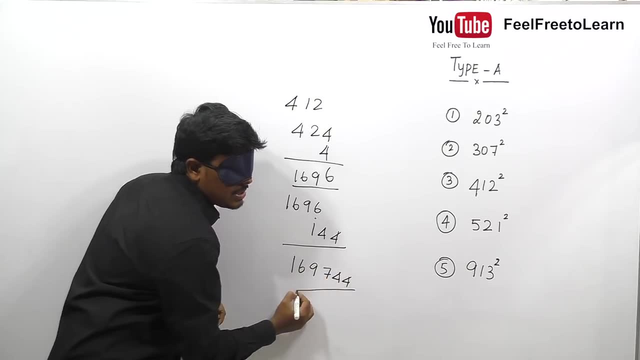 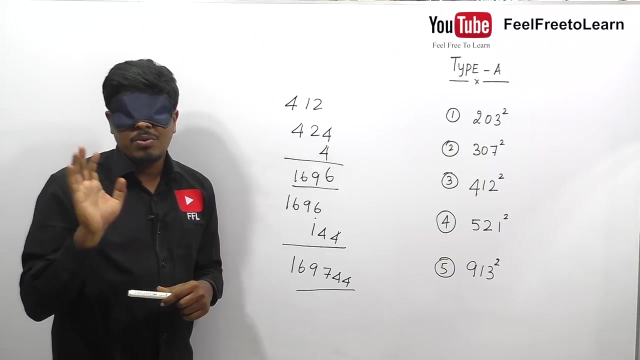 answer should be definitely 6 digit, so 1696, so below 6, 144. so i can surely say that the answer is 169744, so the answer should be 169744. so friends, got the logic. so this is the important thing: that you should know how to square a number. if you practice a lot, then you can surely crack. 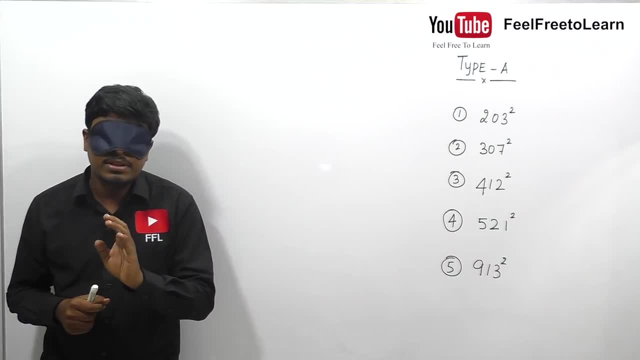 the question, friends, without using pen and paper. now let me move on to the fourth number, that is, you should say whether the answer is 5 digit or whether the answer is 6 digit. i can surely say that the answer must be definitely 6 digit. why? because this 512 is more than 316 whenever. 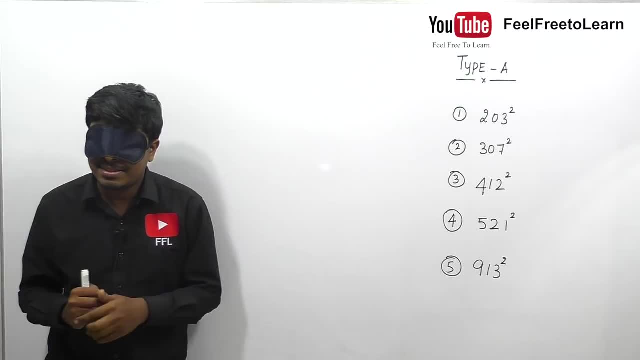 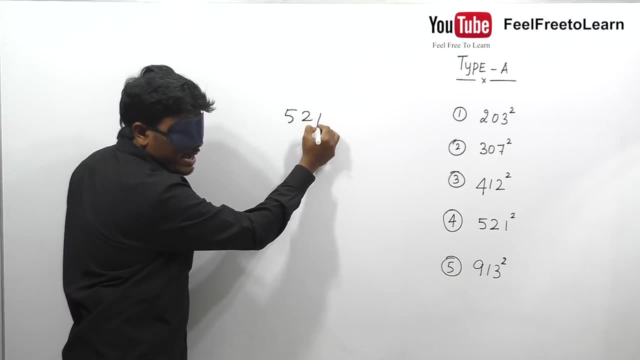 a number is more than 316, definitely the answer should be 6 digit. so, friends, listen carefully. step number one: we found that the answer should be definitely 6 digit, right? so 521 from 500, it is 21 more. so add 21 again to the same number, that is 542. friends, now we need to. 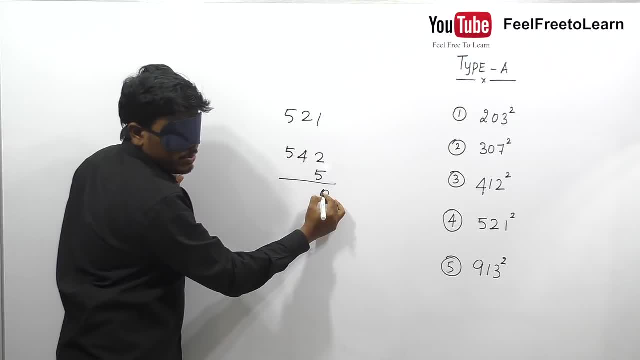 multiply this by 5, so 5 into 2 will be 10. the remainder will be 1. so 5 into 2 will be 1. so 5 was a 20. 20 plus 1 will be 21. remainder will be 2- 5. 5 is a 25. 25 plus 2 will be 27. 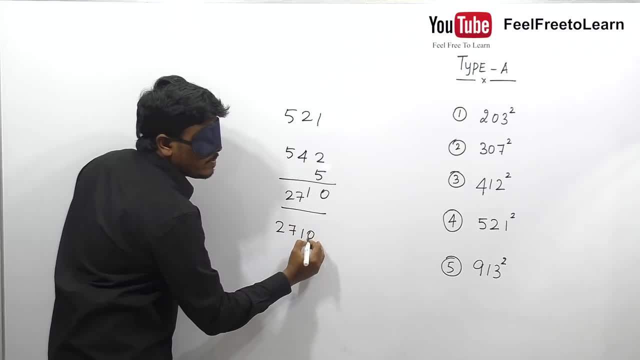 so friends. finally, we got 2710 friends. listen here: when we square, the last two numbers are 21. when we square 21, that is 441. if i write 441 at the last, then the final answer is 7 digit. we know that the final answer should be definitely 6 digit, so write 441 like this 441. so friends. 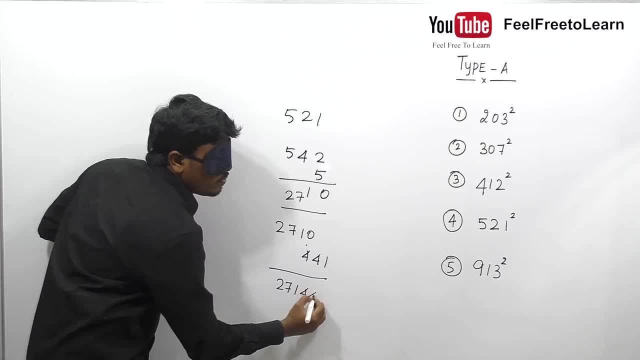 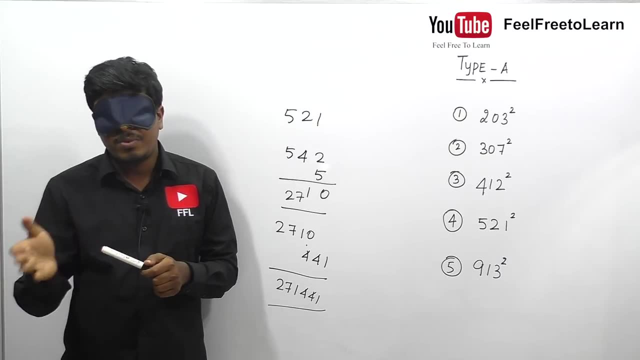 finally, we got the answer: 271441. so this is the answer for when we square a number, that is 521 square, so that is 271441. so, friends, if you apply this logic to all these numbers, if you need to square, that is in the range. 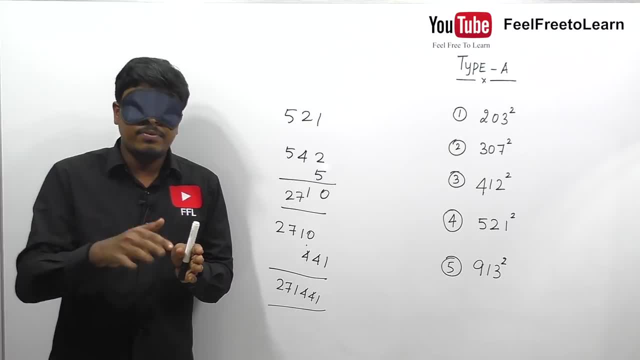 of 1 to 50, right? so 212, 213, 412, 413 or 421, 434? every number can be solved by using a trick. only thing is that- step number one- you should judge whether the answer is 5 digit or 6 digit. if you know this trick, then you can easily solve all the question, that is. 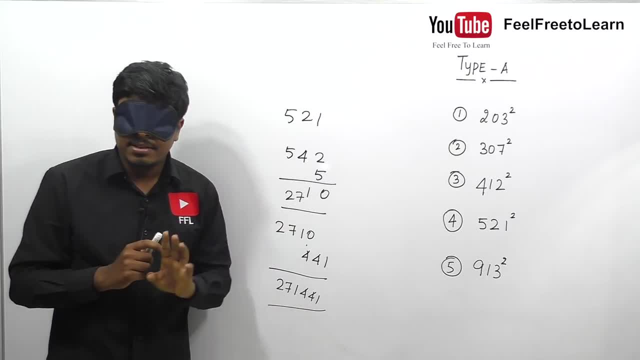 based on type a. so, friends, the last number is 913, square right. so, friends, the same procedure. friends, 913 from 900, it is 13 more. add 13 again to the same number, that is 926. then we need to multiply this by 9. so, 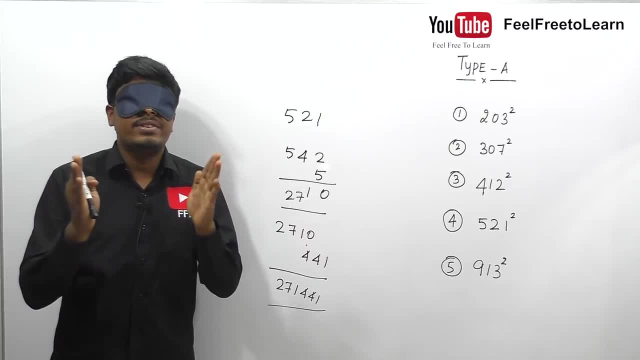 finally, we need to write 169 at the last, so the answer should be definitely a 6 digit. so, friends, i hope that you have enjoyed this type number a, so let me move on to type number b. where type number b? if the number is in the range of 50 to 100? let me move on to the first number, that is. 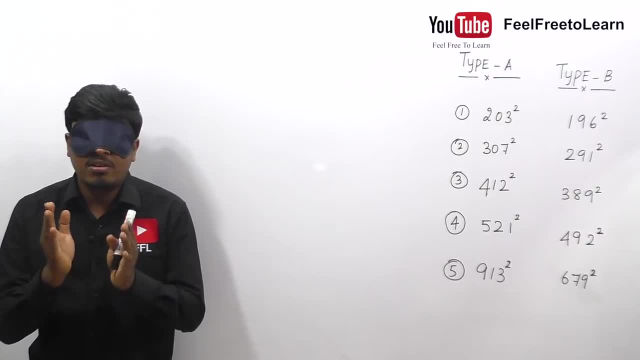 196 square. so friends, listen carefully. so let me move on to type number b. if the number is in the range of 50 to 100, then what the answer must be? 5 digit does ask question. let us see the question is 5. now why 196 is less than 316? yes, because 196 is less than 316, but Every. 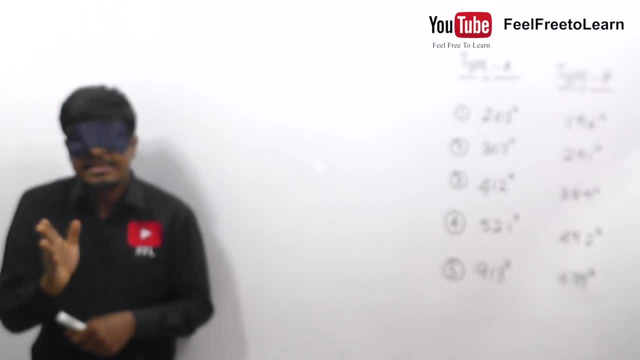 так, wire. there was but the care. if we had the may be 6 or whatever it requires, we need to say whether the answer is 5 digit or six-digit. by seeing a number, i can surely say that the answer must be five-digit. why 196 is less than 316? and now where our number is less. 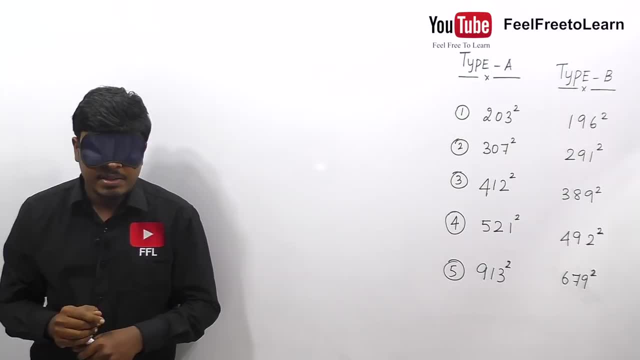 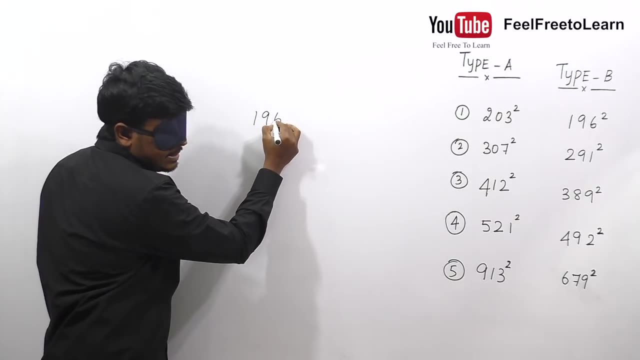 than 316, then definitely the answer must be 5 digit. so, friends, listen carefully. i'm just going to teach you slowly, right? so, friends, listen. here we are just going to square what is 196. so, friends from 200, listen here, friends from 200, it is four less. friends got the point. 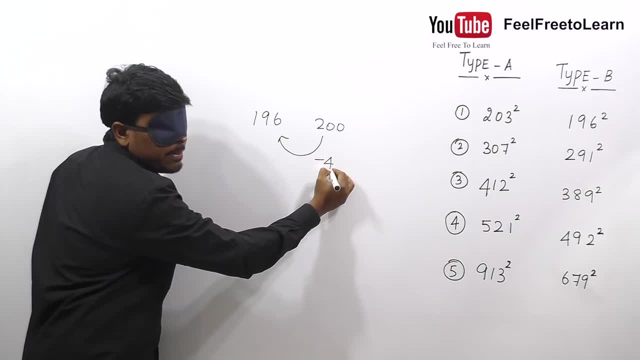 from 200 to keinen less than now, it is 4. 0 is just 4 to minus. oike, i have пл kopay nagar. 200, it is 4 less. so i am just going to subtract 4 in the given number. 196 minus 4 will be 192. 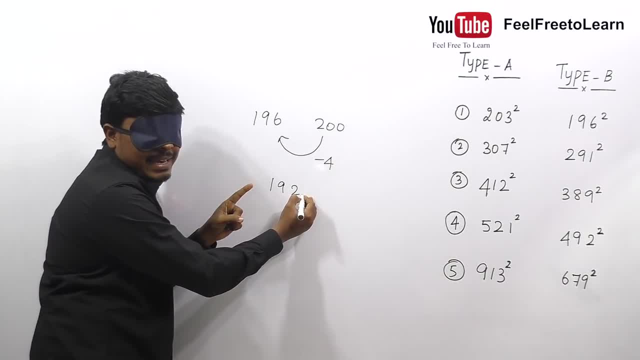 so friends got the point. this is the step number 1. in the first case, right in type a from 200 it is 3 more. so we add 3 again to the same number, that is type number a. but in this type number b from 200 it is minus 4 less. so we are just going to subtract minus 4 in the given number, so 196. 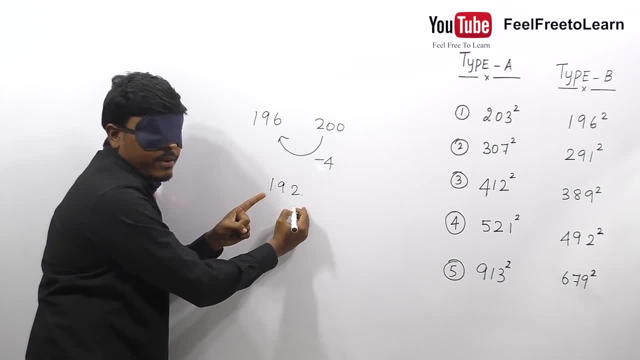 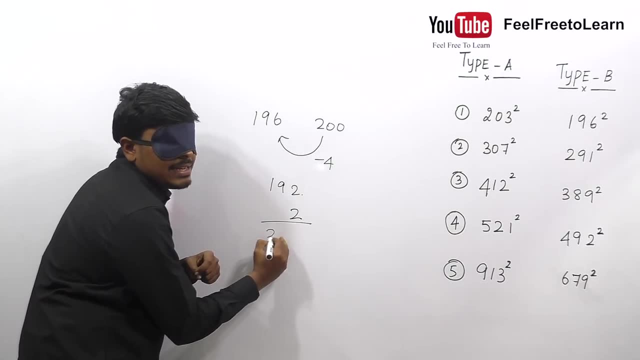 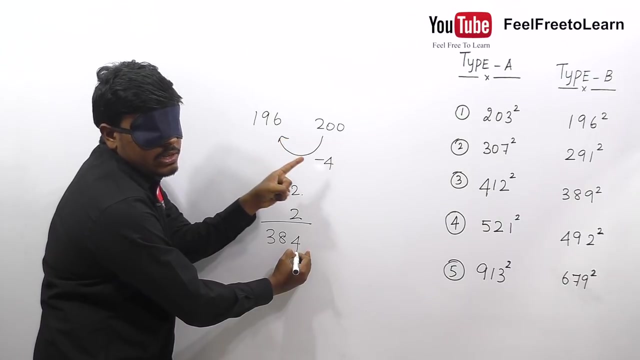 minus 4, the resultant will be 192. so, friends, from 200 we have calculated, so the base number is 2. we need to multiply this 192 into 2, so finally we can say that 384, so friends, finally we got 384. friends. listen here: from 200 it is 4 less, so 4 square that is 16, so finally we can say the answer. 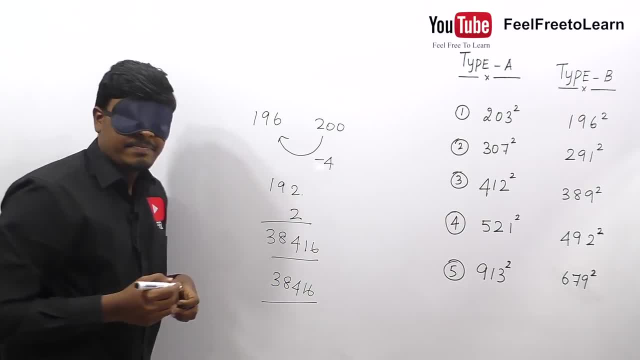 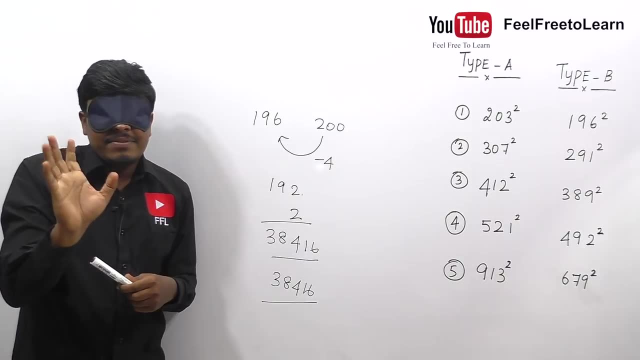 as 38416. so this is the answer. so, friends, 38416. friends got the point. friends, just just listen carefully- from they have given a number: 196 from 200. it is 4 less. first of all, we have subtracted 4, that is 192 from 200. we have calculated. so we need to take base number as 2. so 192 into 2, that is 384. 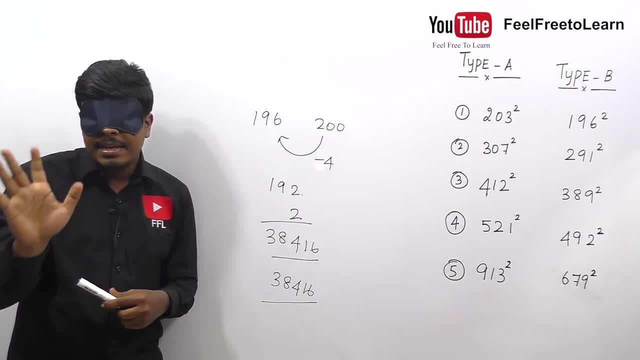 finally we got 3 digit. we know that the answer should be definitely 5 digit. listen here, friends, from 200 it is 4 less so 4 square, that is 16. so finally we got the answer as 38416 sum number 2, that is 296. 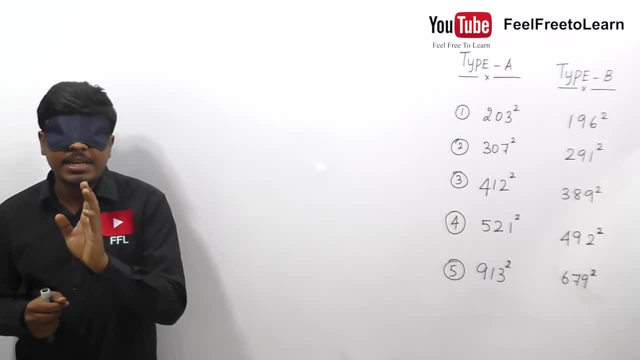 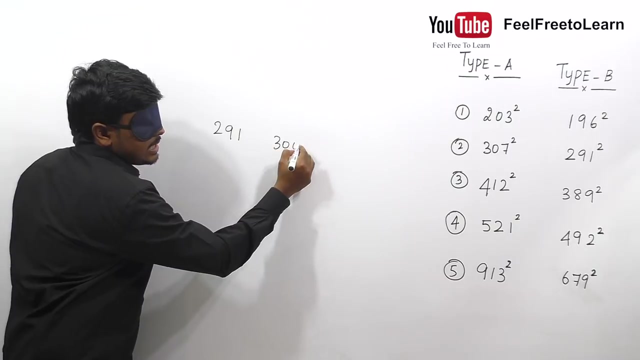 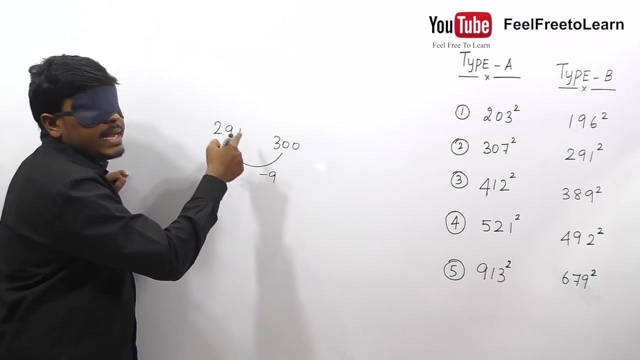 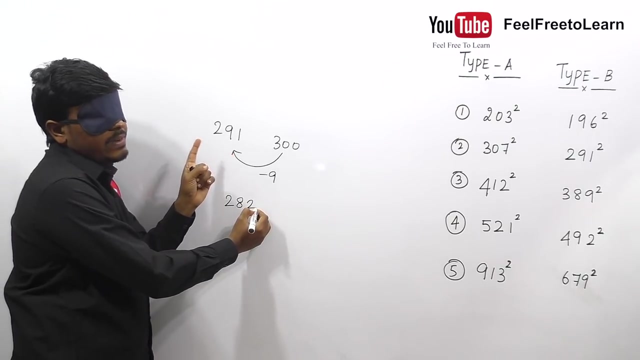 297, the answer should be 3 over 2, 21 square. so one step, number one. always remember that we need to say whether the answer is 5 digit or 6 digit. we can surely say that 291 is the number that is less. friends got the point. from 300, it is 9 less, so we are just going to subtract 9 in the given number. 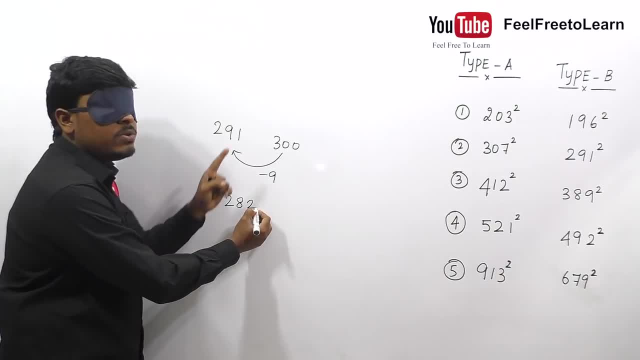 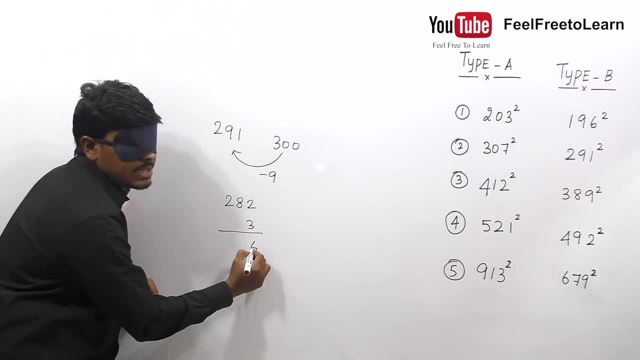 that is 291 minus 9 will be 282. we took the base number as 300, so we need to multiply this by 3. so when we multiply this by 3, 3 into 2 will be 6, 8. 3 is a 24. the remainder will be 2. so finally, 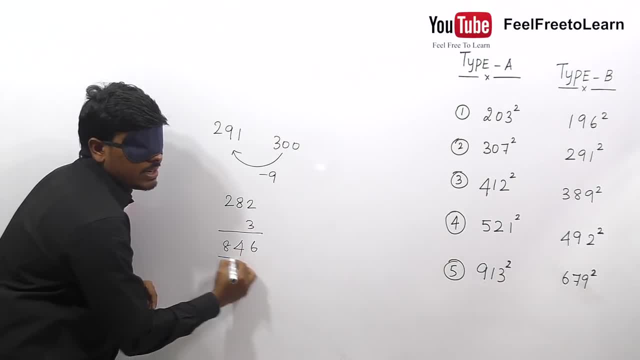 we can say that 3 into 2 will be 6, 6 plus 2 will be 8, 8, 46. so, friends, we got 8, 46. listen here, friends: from 300 it is 9 less, so 9 square will be 81. so finally, we can say that the answer is 8. 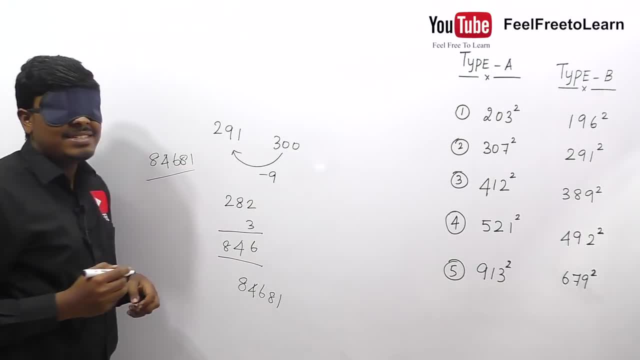 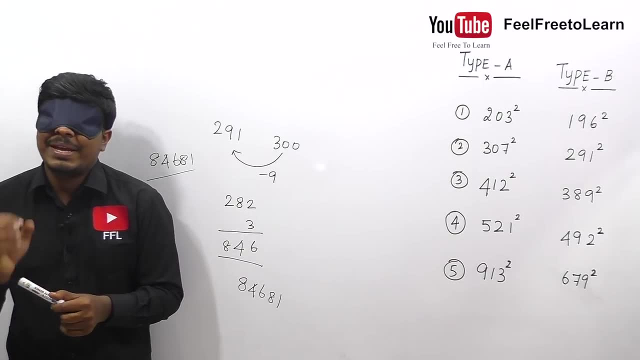 4, 6, 8, 1. so finally we got the 5 digit, that is, 8, 4, 6, 8, 1. so, friends, this is the concept. friends, right, though it is a very big number, you can surely crack the question by using this method, right? 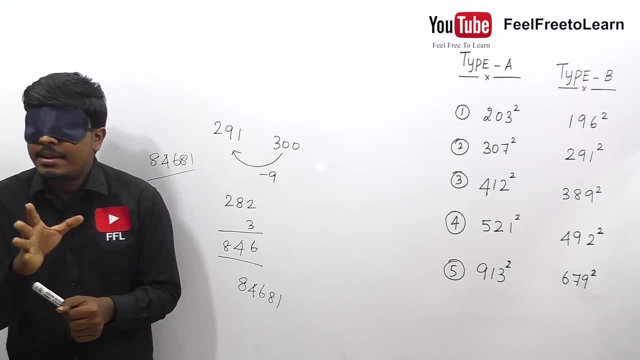 practice a lot, practice, practice, practice a lot daily at least a number, 10 or 20 numbers. you can also close your eyes and you can also say the answer right. so, friends, what are all the things we added? step number 1: we have just found whether the answer is 5 digit or 6 digit from 300, it is 9. 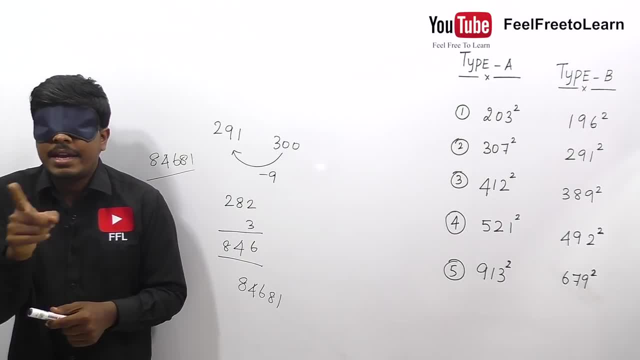 less. so we need to subtract 9 in the given number, that is, 291 minus 9, 282, so 282 into 3. why? because we have to base number as 300, so we need to multiply this by 3 and we multiply this by 3. 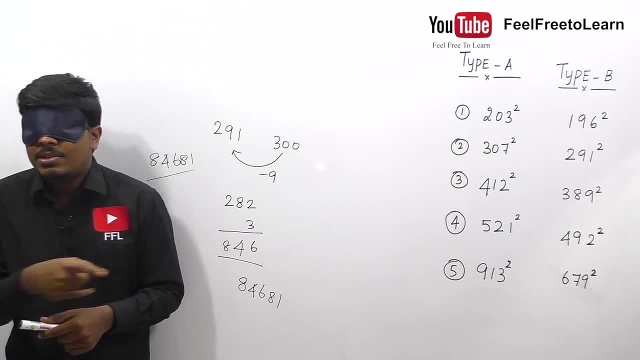 so 8, 46. we know that the answer should be 5 digit, so last number is from 300. it is 9 less, so 9 square will be 81. so finally we can say that the answer is 8, 4, 6, 8, 1. 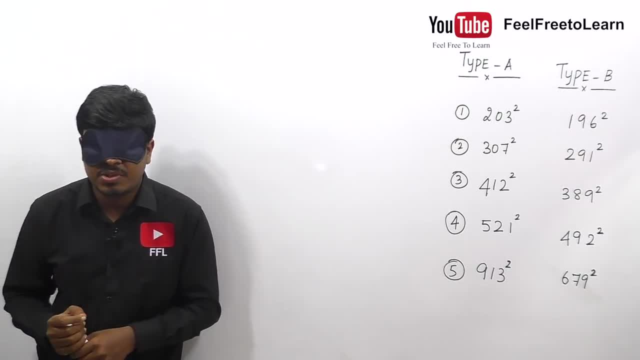 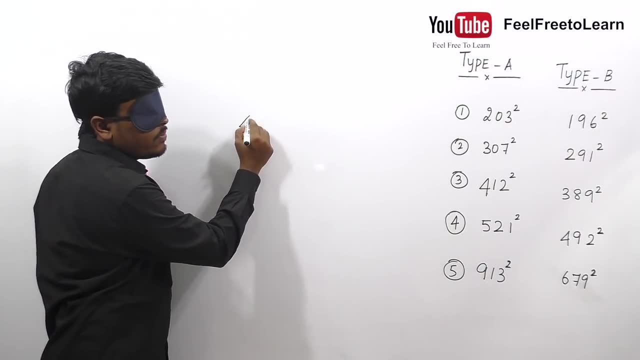 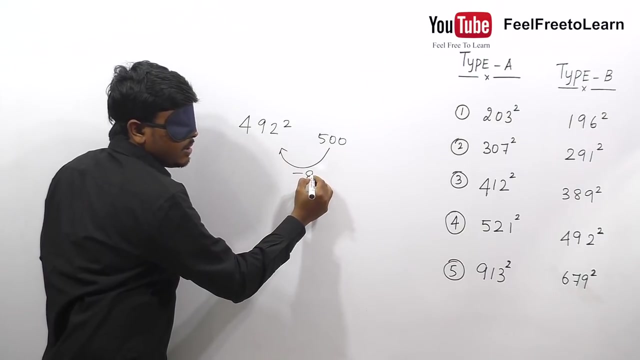 now let me move on to the huge numbers. right, that is 492 square. so, friends, we are just going to see what is the answer for 492 square. so, friends, listen carefully. apply the same concept, right? so 492 square. so, friends, we can surely say that from 500 it is 8 less. right, we are just going.